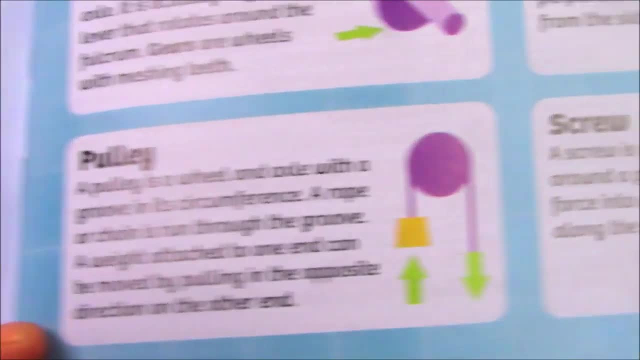 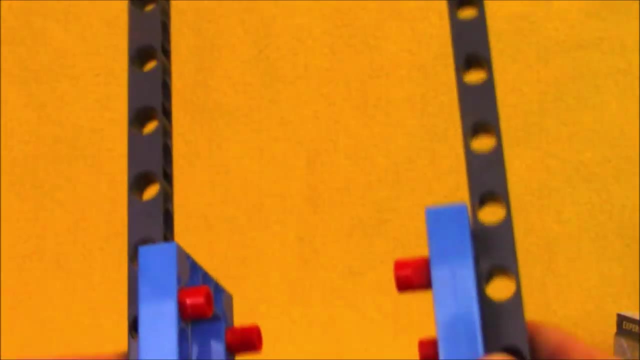 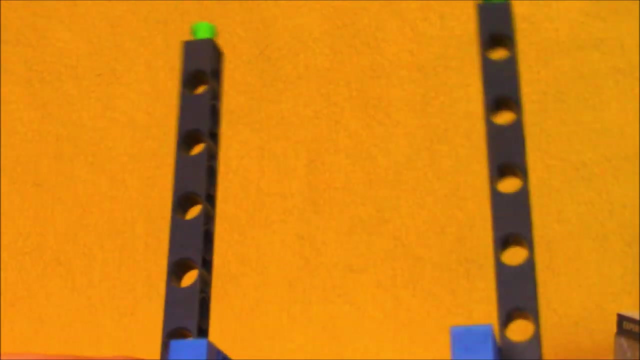 This stem kit covers levers, wheels and axles, pulleys, inclined planes, wedges and the screw. The parts and pieces that you use to build the different experiments are very sturdy. they are pretty easy to assemble. they remind me of some classic building toys. 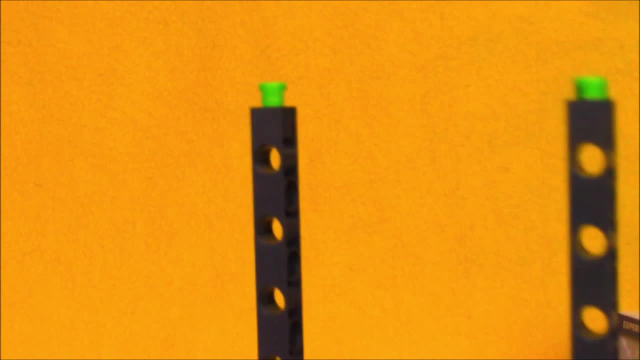 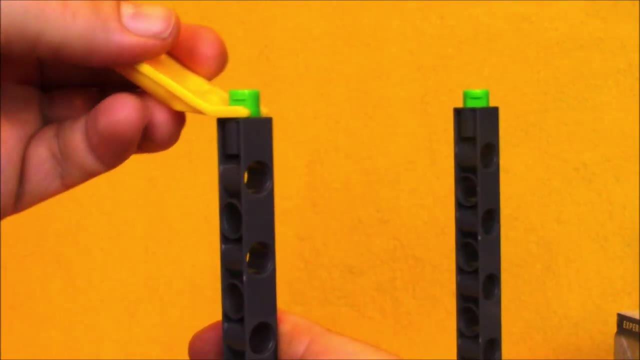 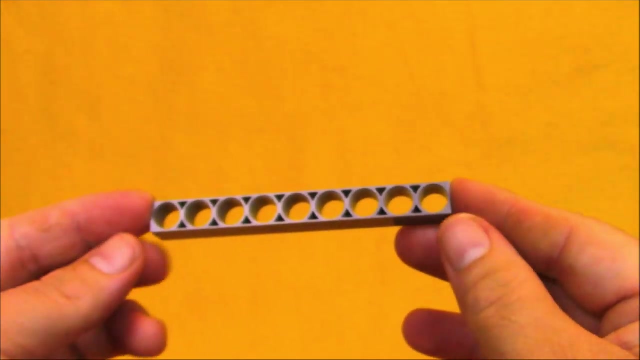 but they're a little bit different. they're a little bit unique. I think it's really funny that you get your own lever with the kit for separating pieces. it's very appropriate for this stem simple machines kit. The set includes some frame pieces as well as some rods that have a series of holes in them. 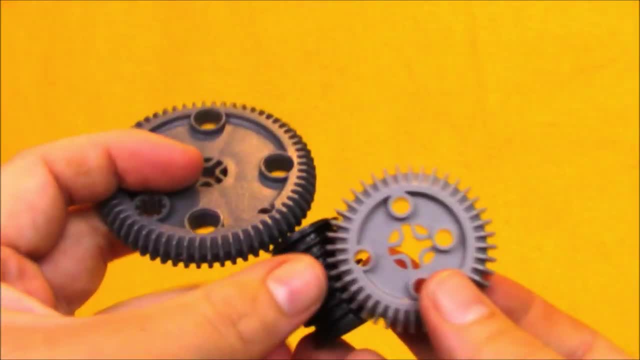 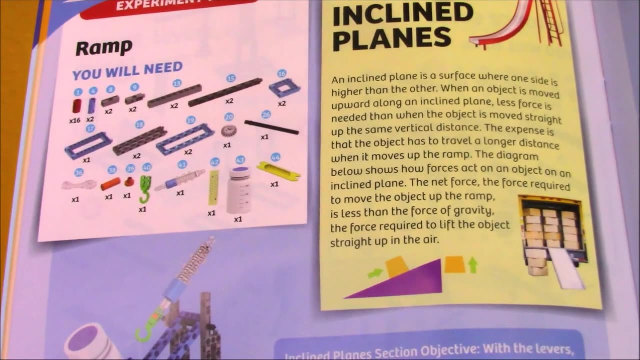 there's multiple different colored connector pieces in different lengths, different types of gears. you can assemble your own pulleys. With each one of the experiments you get a little science lesson that explains what's going on with this simple machine. it shows you all the parts you're going to need. 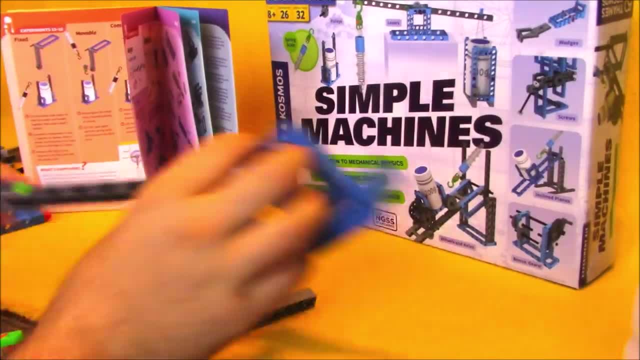 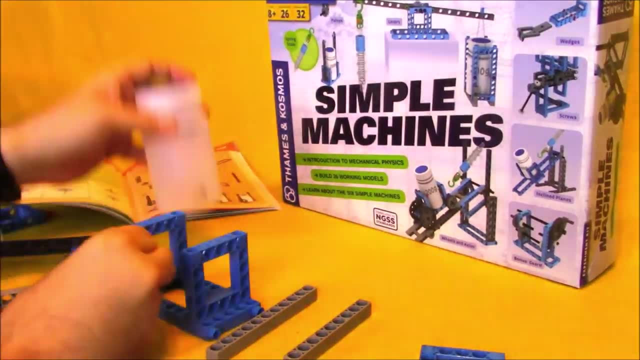 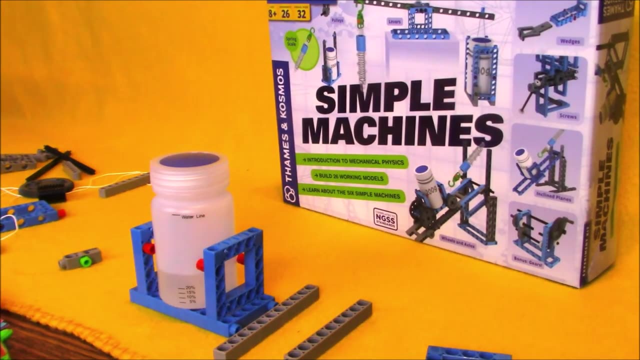 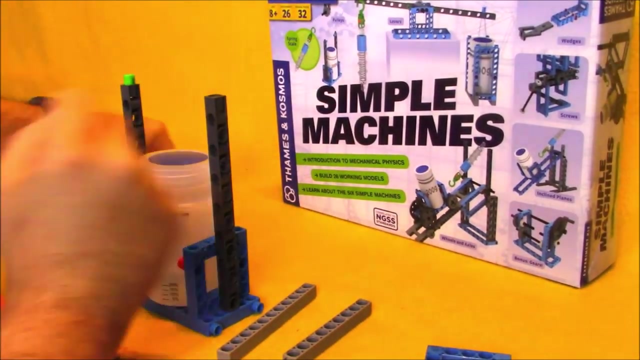 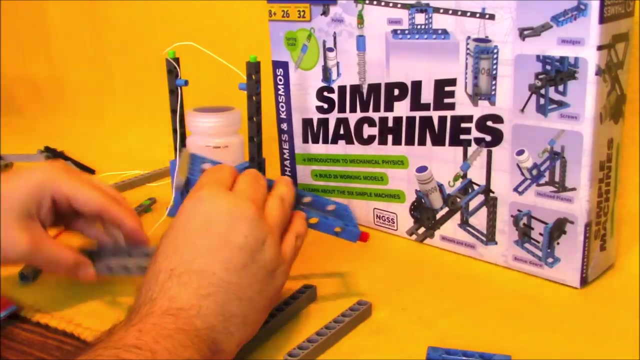 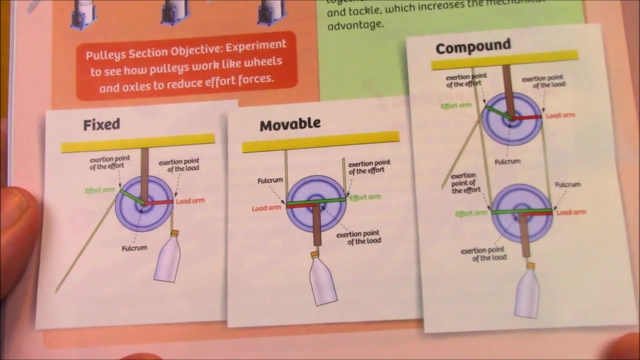 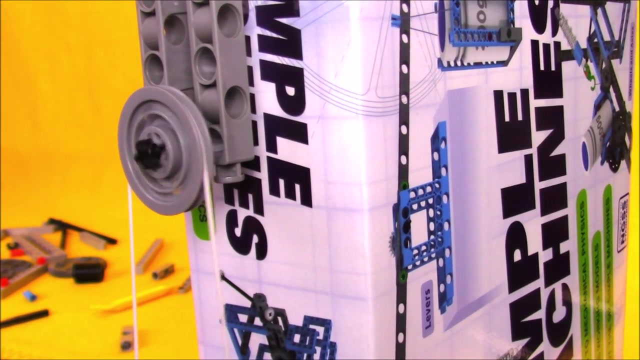 and then it has. you build the system. Now let's take a look at the device. In the case of the pulley, you build one basic setup, but there are some variations. Time to operate a fixed pulley. Here's the movable pulley in action. 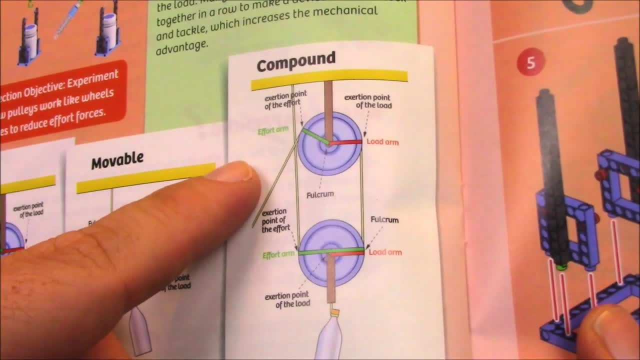 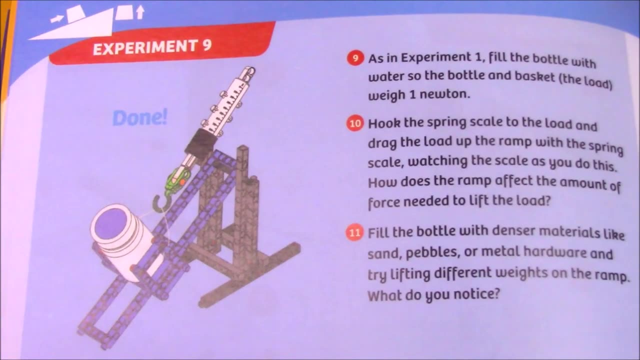 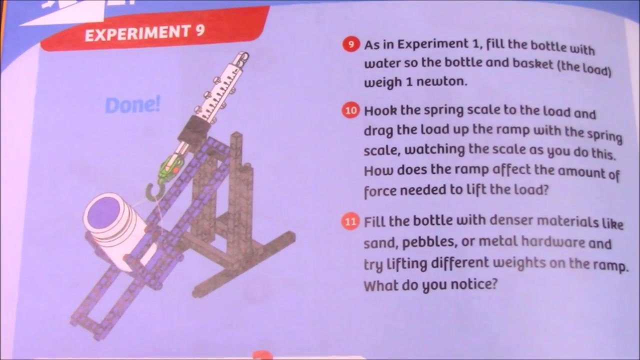 I assembled the compound pulley and it was pretty neat, but I had a hard time filming it. This one would definitely be easier with a friend's help. Most of the experiments have you use the spring scale to take some measurements and you can use this information to gain some insight into how much work you're actually performing. 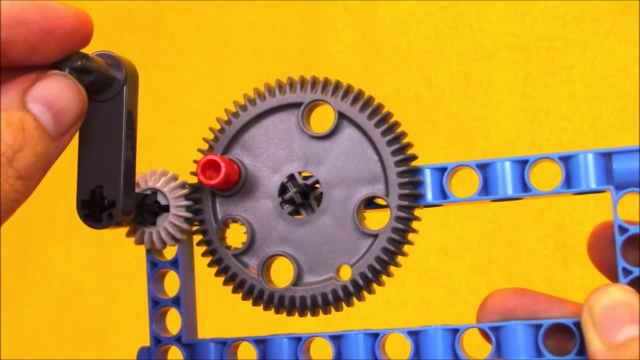 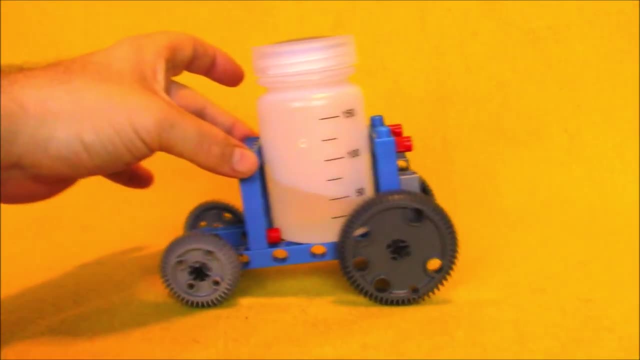 You can do experiments with gear ratio. Watch how many times I have to crank the handle to get the red peg to go all the way around. One, two, three. This little buggy is part of the wheels and axle. experiment number 11 and 12.. 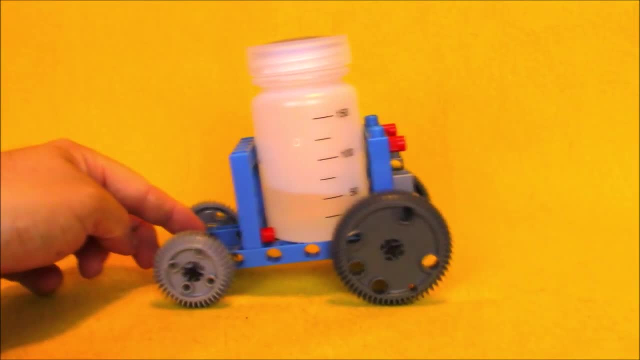 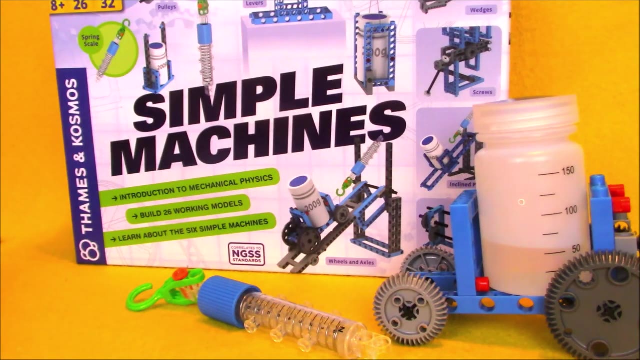 You can take force readings on this to see how much effort it takes to move this. then switch out the wheel diameters and see how that affects the way the vehicle rolls. The Simple Machines STEM Experiment Kit is a lot of fun to work with.